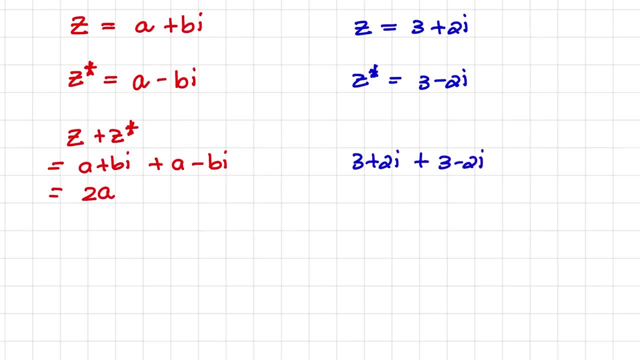 its conjugate, which is 3 minus 2 i, and that is equal to 6.. In our second example, let us say we have a complex number and we want to subtract its conjugate from it, So that will lead to a plus b i. 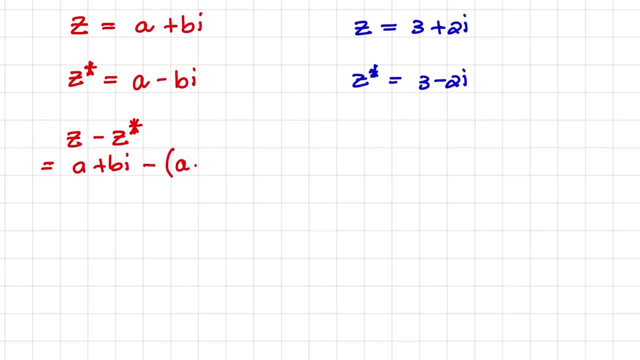 minus and then in parentheses a minus b i, And when I simplify that will be a plus b i minus a plus b i, which is equal to 2 b i. So let us look at a practical example again of subtracting the conjugate from a complex number. So we have 3 plus 2 i minus 3 minus 2 i. 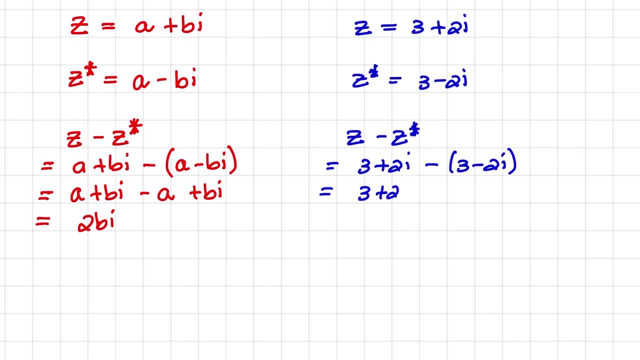 And when I simplify it will be 3 plus 2, i minus 3 plus 2, i So remember the sign change and that leads to 4. i Notice it is not equal to 4. i squared, We are simply adding the coefficients. 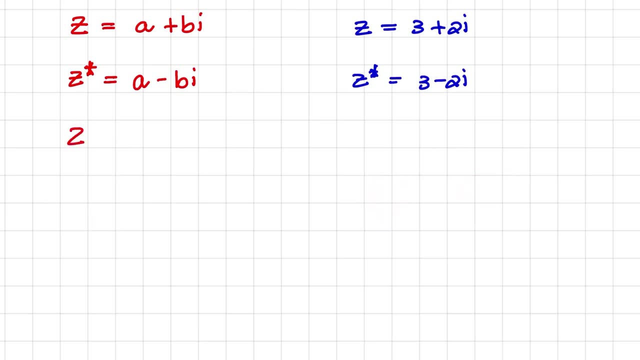 together. Let us see what happens if we multiply a conjugate with a complex number. So in this example it will be a plus b i minus 3 plus 2 i, And when I simplify it will be 3 plus 2 i minus 3 plus 2 i. 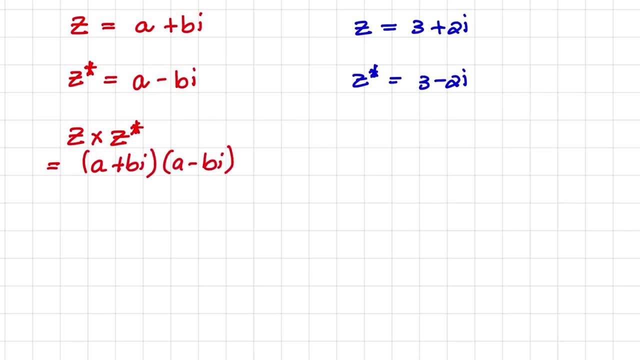 Now let us take an example of subtracting the conjugate. So let us say: i is equal to b i times a minus b i, And when I simplify, that leads to a squared minus b squared, i squared. But remember that i squared is equals to negative 1.. Because i represents the square root of negative 1, and when I square that, 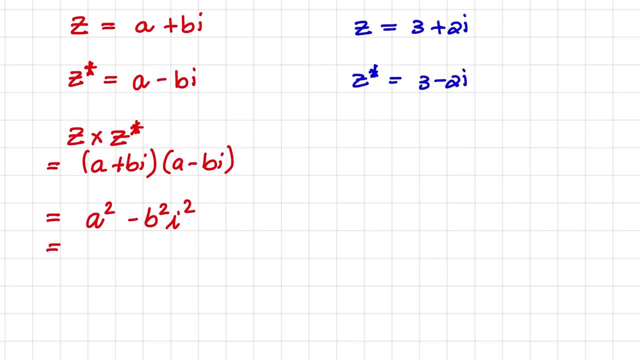 it leads to negative 1.. So if I simplify further, I have a squared plus b squared. So let us look at at our example again. we have z times its conjugate, where z is 3 plus 2i times 3 minus 2i. 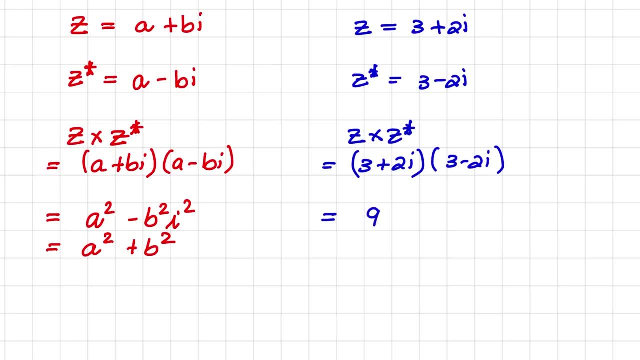 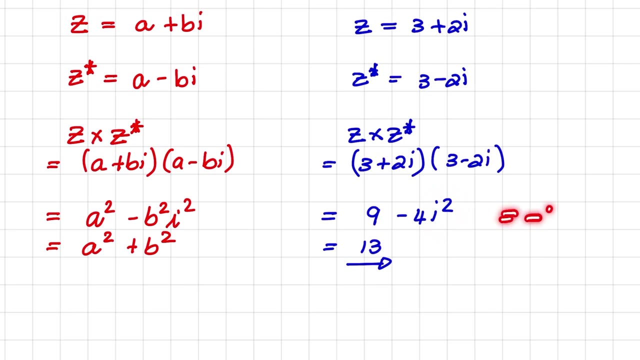 and when I simplify that, that leads to 9 minus 4i squared, and if I simplify further, it becomes a real number where it's simply equal to 13.. Remember that i squared is equal to negative 1, so it's 9 minus 4 times negative 1, which is 9 plus 4, and that becomes a real number of 13.. 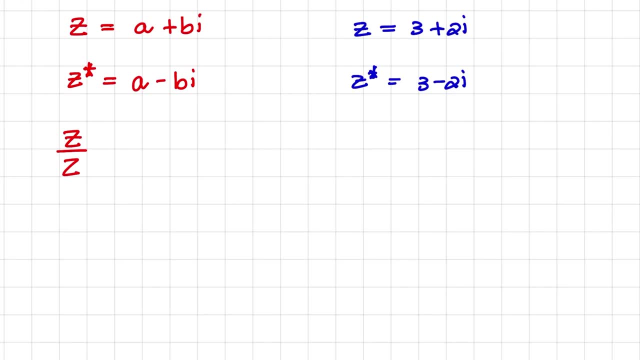 And lastly, let us look what happens if we divide a complex number by its conjugate, so that'll be a plus bi divided by a minus bi. but remember, in order to simplify this division, I need to multiply the numerator and denominator with the conjugate of the denominator, so that'll be a plus bi. so in 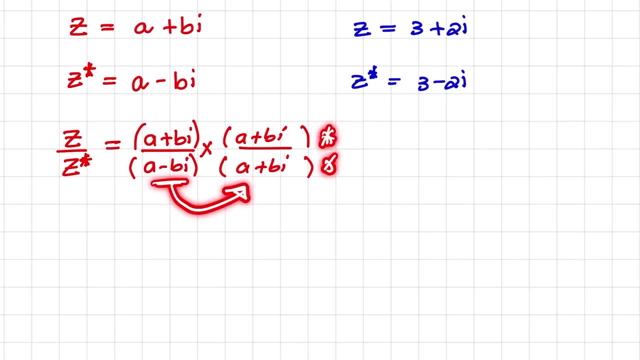 effect I'm multiplying the numerator and denominator with the conjugate of the conjugate, which is the original complex number. So let us again look at our practical example. here we have z divided by its conjugate, and that'll be 3 plus 2i divided by 3 minus 2i. 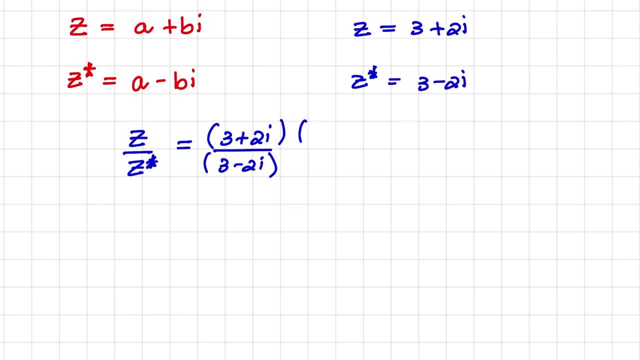 And in order to simplify this fraction, I would multiply both the numerator and denominator by the conjugate of the denominator, so that is 3 plus 2i. and when I simplify that, remember, I simply need to multiply out the parentheses as I would do normally in algebra. So in the numerator I have. 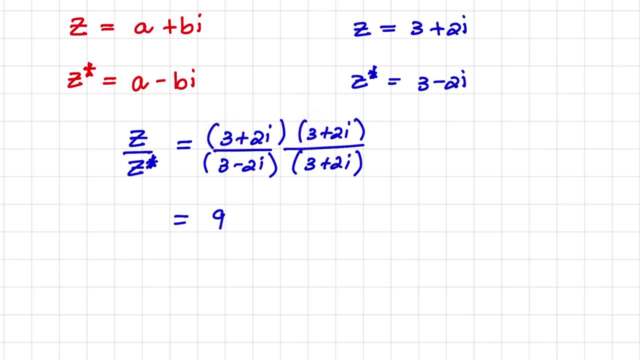 3 times 3, which is 9 times 3 times 2i, which is 6i. So now that I've used this form, I simply need to multiply both the numerators and denominators. So in the numerator I have 3 times 3, which is 9 times 3 times 2i, which is 6i. 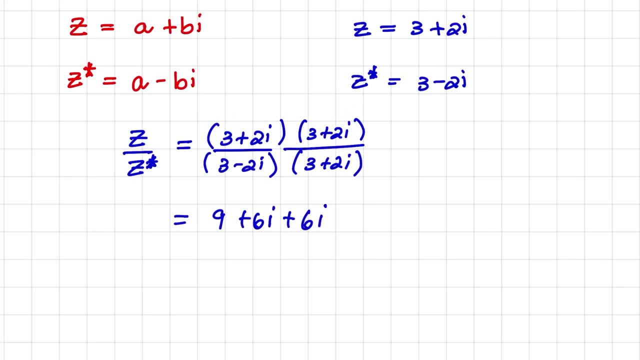 plus 2i times 3, which is 6i plus 4i squared. remember that i squared becomes negative 1 over 3 times 3, which is 9, and then the middle terms will cancel out. so it's minus 4i squared. 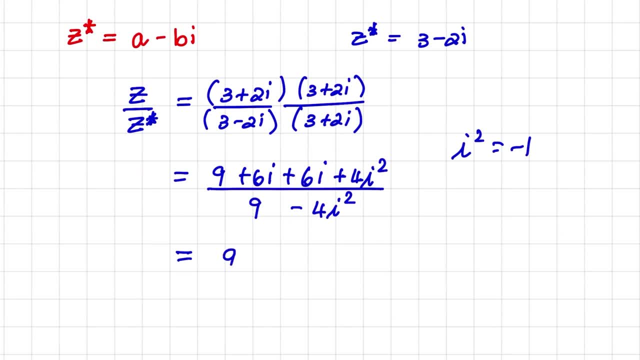 and if i simplify further, i have 9 minus 4 plus 12i, where the minus 4 comes from 4 multiplied with negative 1, so it's 9 minus 4 and then 6i plus 6i is 12i and in a denominator, 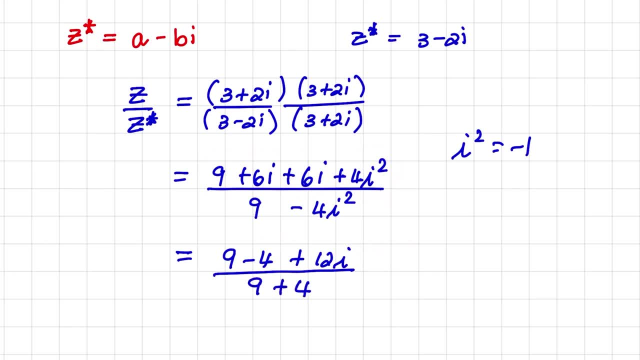 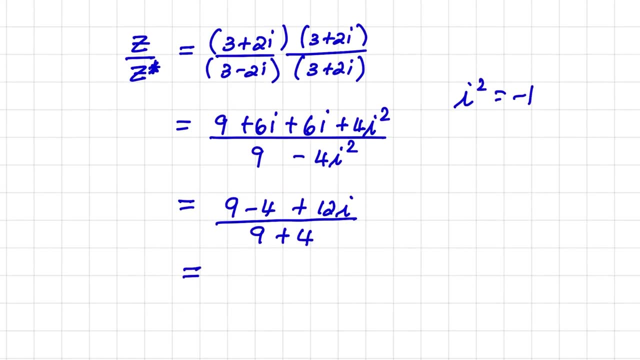 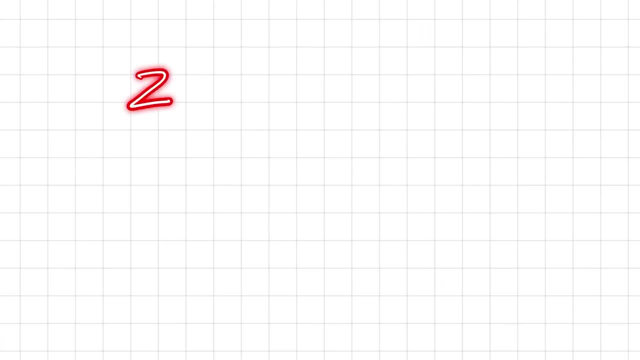 i have 9 plus 4, where negative 4 times negative 1 becomes plus 4. so if i simplify, i have 5 plus 12i over 13. so there we have it. we have learned what will happen when we add the denominator to the denominator. so we have 9 plus 4 and then we have 9 plus 4.